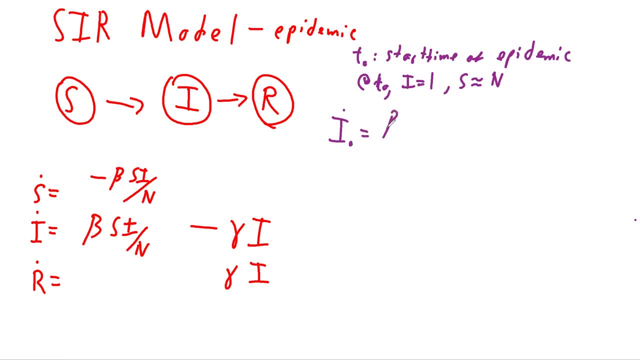 is going to be equal to beta S I over N minus gamma I, But because of our assumptions of what happens at T-naught, I is just one, So that goes away. That goes away. And similarly, S is approximately N. And look, that means we get to rewrite this as N. 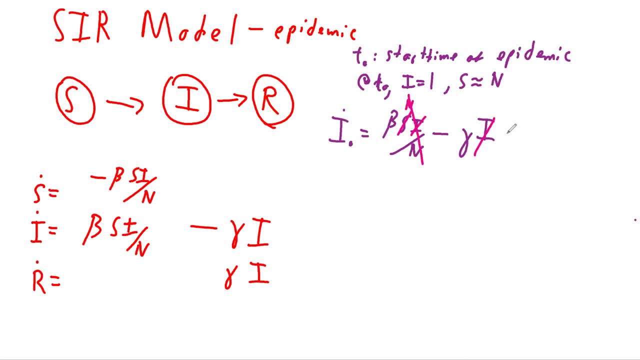 And N over. N is one, So this just goes away. And what are we left with? We're now left with beta minus gamma. Well, that's easy. It's also very important and extremely convenient. This is going to look a little weird, but humor me. 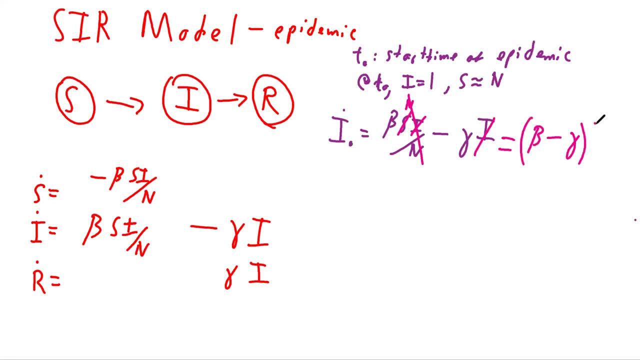 What I'm going to do next is I'm going to take this and multiply and divide by gamma. for a very specific reason, Because what this comes out to then, if I do that and I distribute as I want, is I'm going to get a term: gamma times beta over gamma minus one. 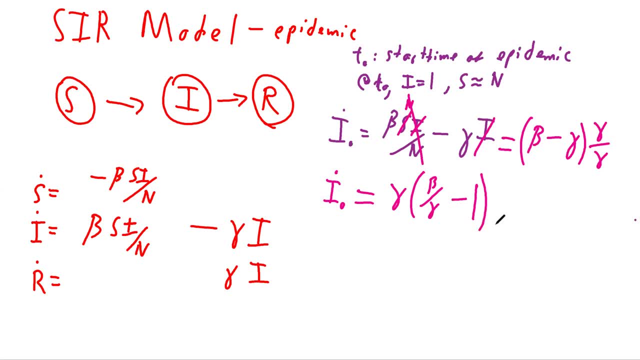 That was set up intentionally. Okay, Why? Because this property right here, this value is R-naught. You said this is equal to gamma R-naught minus one. And look at what this is saying here. This is saying that the rate of change 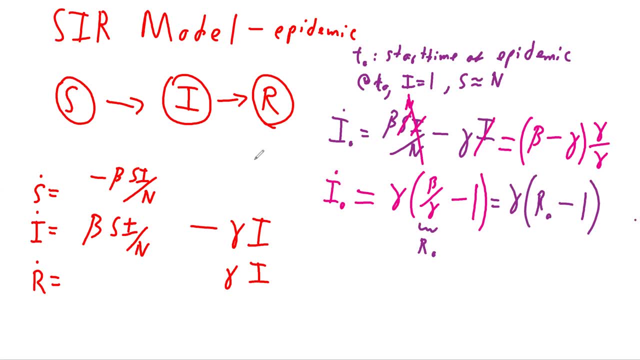 the number of people that are added or subtracted to the infected population at the very first time- initially, as the epidemic is just about to grow because we only have one infected person- is determined entirely by this equation: gamma beta over gamma minus one. 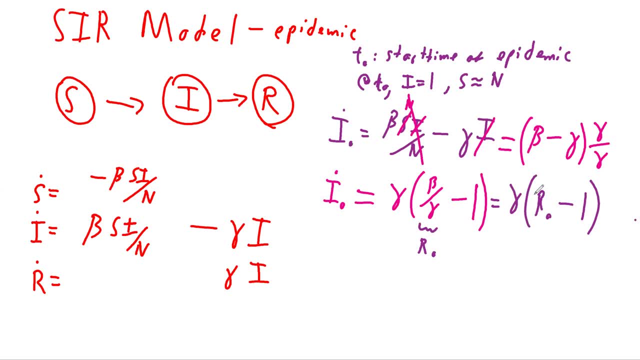 And that is that beta over gamma is termed as R-naught. If you look at this, you can see, then, that for an infection to be positive, for the rate of change here to be greater than zero, right For new people to be added to this pool. 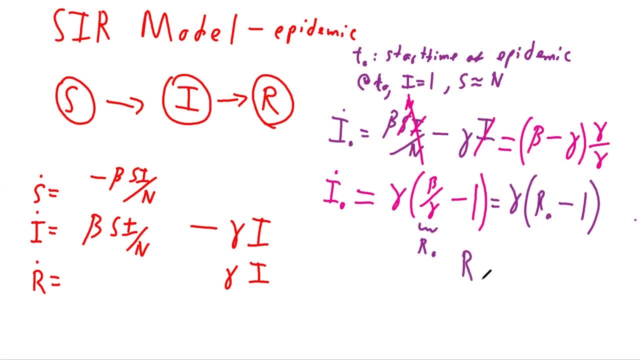 R-naught here has to be greater than one, And if it's greater than one you have an epidemic. That means that in time, as the dynamical system evolves across time, the number of people in I are going to grow If R-naught is less than one. 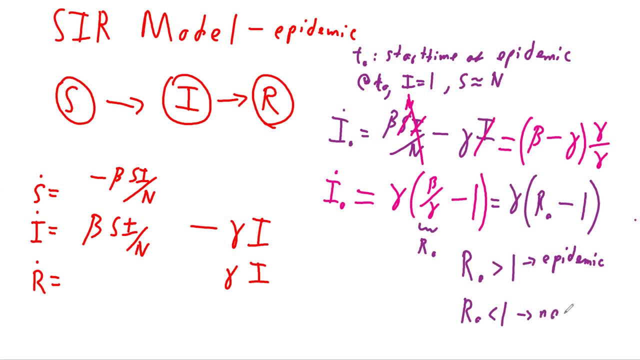 you will not have an epidemic. You will not have an epidemic. You will not have an epidemic, No epidemic. Why? Because the number of people that are being added right, The rate of change of the infected population, is going to be negative. 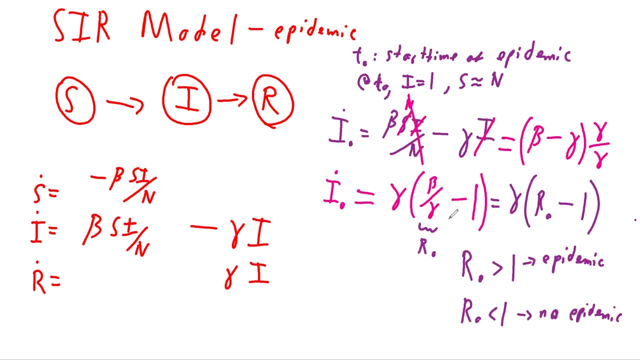 And so, even from the very first case, the infected pool is going to fall and you aren't going to get a spread of COVID-19.. The disease- This term are not- is critically important in epidemiology and health policy. It's called the basic reproductive. 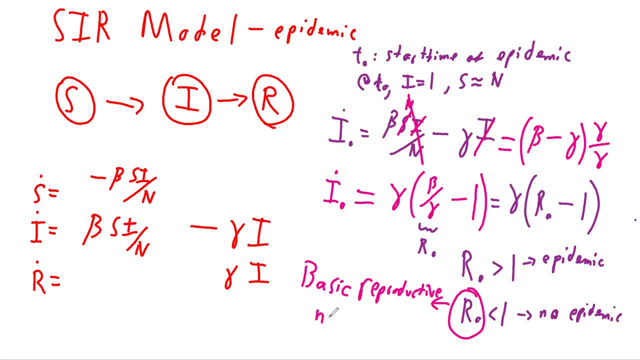 number of, of, of, basically of of of an infection, and epidemiologists and people that that set health policy are very concerned about. what this are not is Because if it's greater than one, suddenly that particular type of disease is a health risk in populations. If 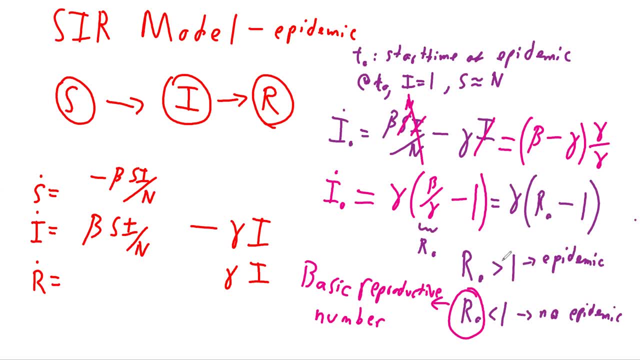 it's less than one, they tend not to care. How much greater it is than one is also of serious concern. If this number is extremely large, like in the case of, say, measles, which is something on the order of like 13 or 15,, then that particular disease can spread like wildfire. 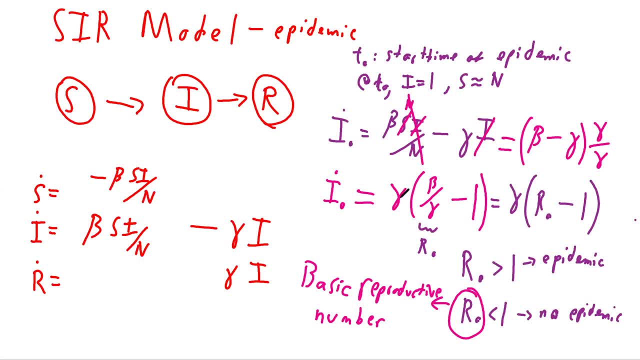 throughout a population. Because what is it saying? It's saying that for every person that's infected, our- not number of additional people are expected to be infected by that individual person. So it's the rate at which it's how many multiples of people are infected, based on every individual. 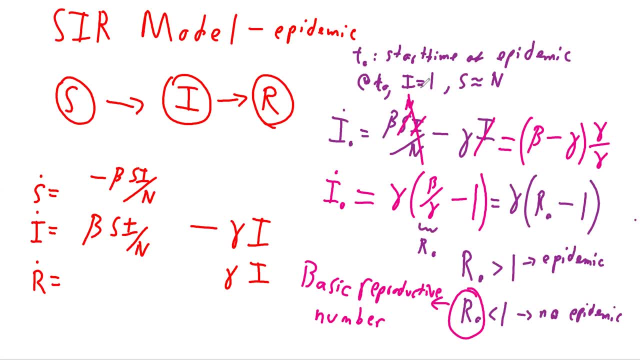 index case, So measles spreads really quickly, Other diseases not so much. We're really terrified about Ebola, And we hear a lot about that often in the news, but it turns out it's R-naught is on the order of like two or three, And so it doesn't really pose that much of a health risk.